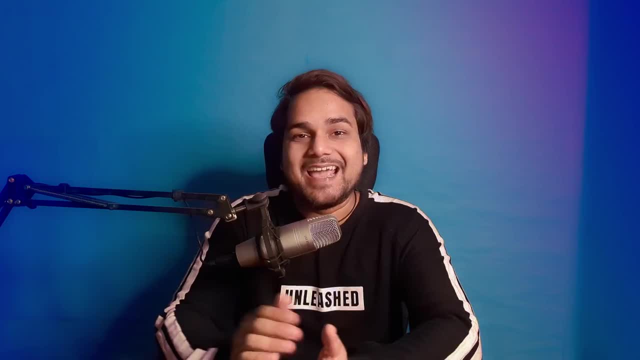 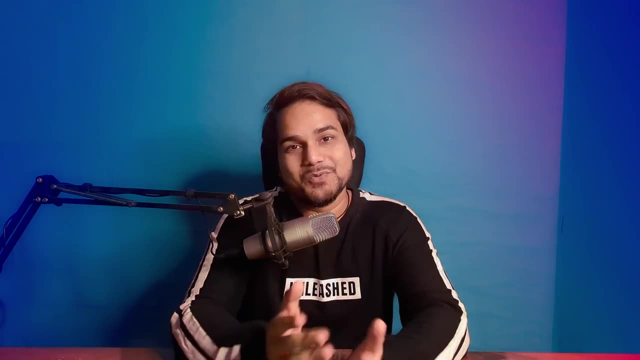 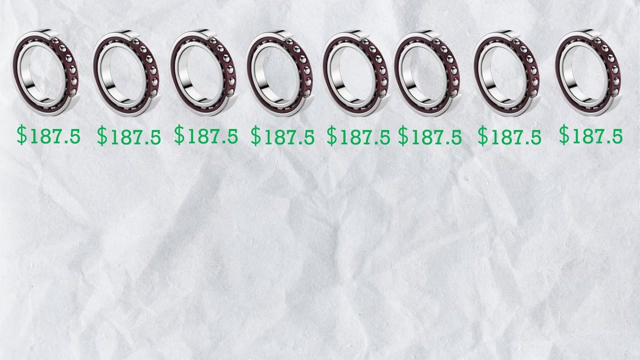 the bearing can be seized just in few minutes at high speed. and this is my own experience. yes, my own designed bearing block bearings had failure twice. eight pieces of angular contact bearing had been failed and the total cost was around fifteen hundred dollars. it's 1.2 lakh rupees. so we will discuss all these advanced things, so you 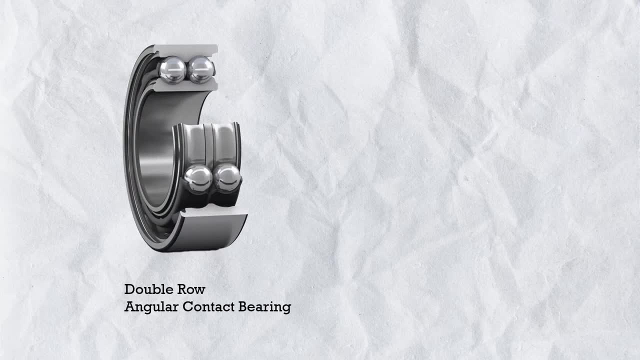 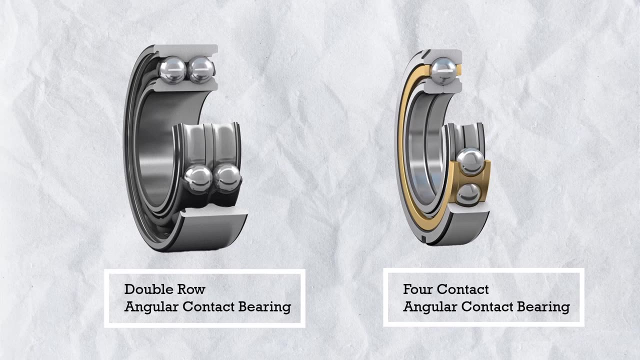 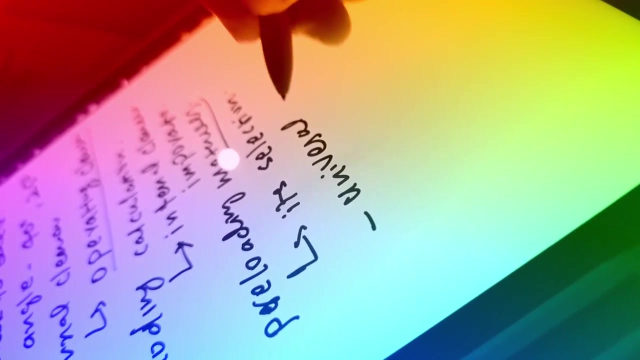 will be able to avoid such disaster. and there are also two more types of angular contact bearing: double row angular contact bearing and four contact angular contact bearing. so initially video length was going more than 40 minute because there are so many terms and independent topics and i don't want to compromise on any topic because of the video length, so i have 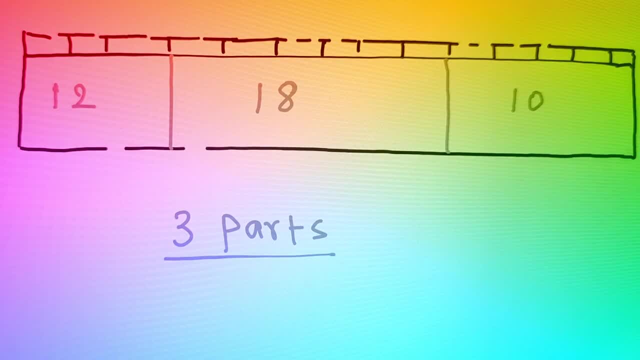 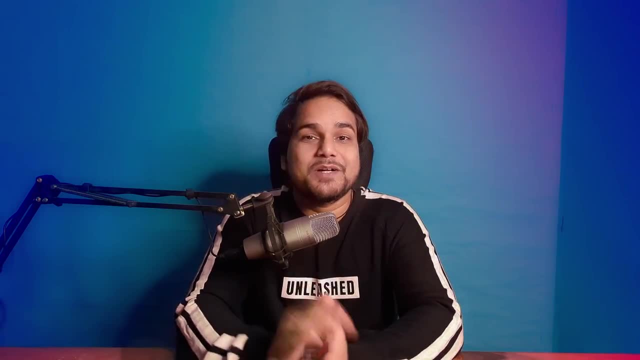 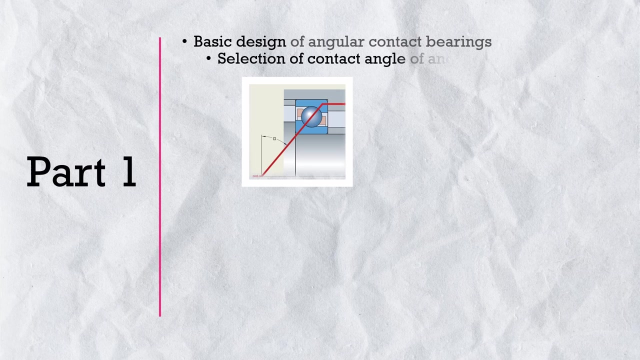 added this angular contact bearing video into three parts, but it's all because of you, so you can easily navigate and watch each topic separately as per your need. so in this first part we will mainly focus on basic design of angular contact bearings, like selection of contact angle of angular 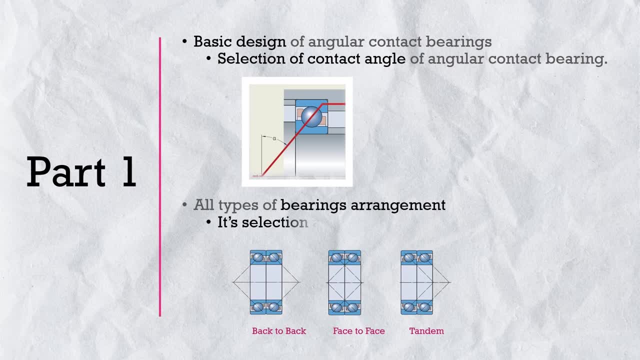 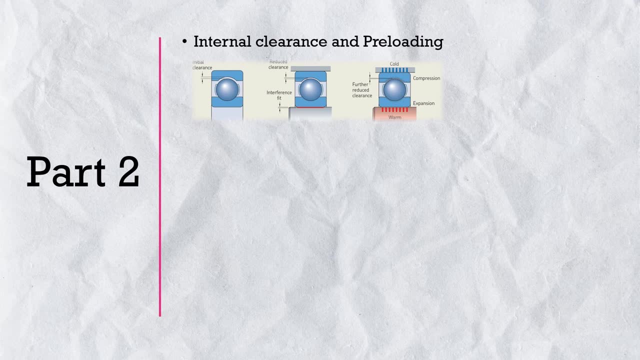 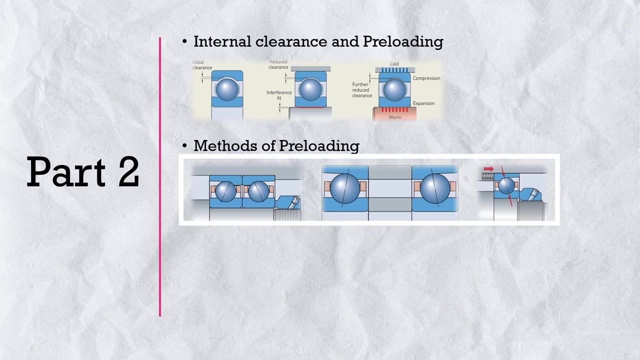 contact bearing all types of bearing arrangement and their selection as per the application. and in the next part we will learn angular contact bearing internal clearance and the preloading, like how to do the preloading, what are the methods of preloading and which method is more suitable for which application and, most importantly, how much preloading is suitable for. 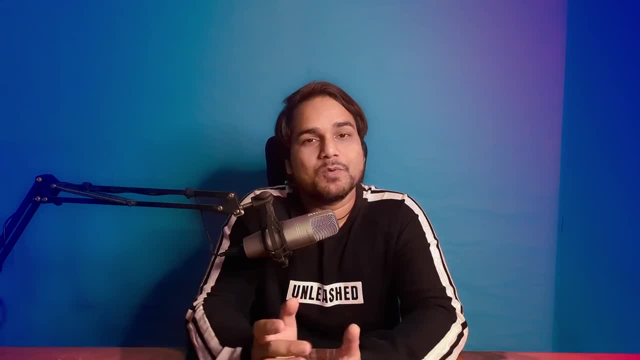 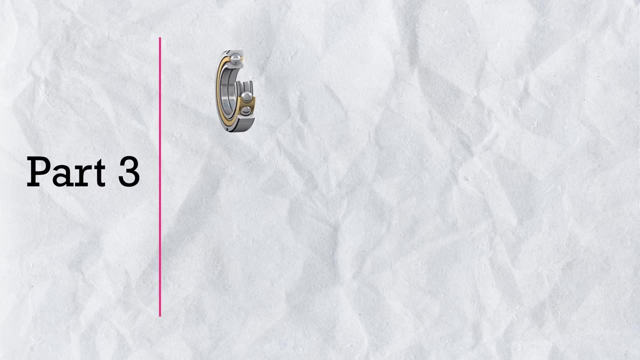 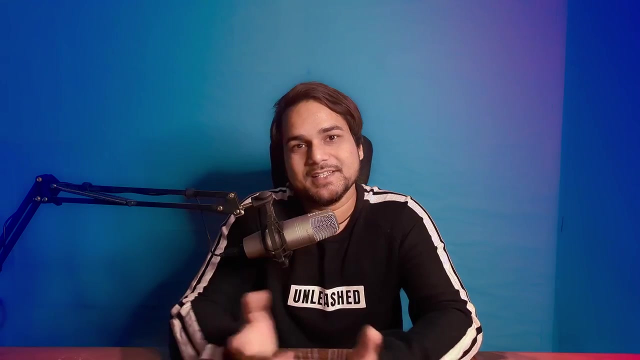 which type of application and what is the alternative of not doing preloading manually, like universal meshed bearing. and in the third part we will focus on rest of two other types of angular contact bearing and their application. also we will cover taper roller bearing. so let's start from very basic. so, as we have seen in the previous part of this bearing series for 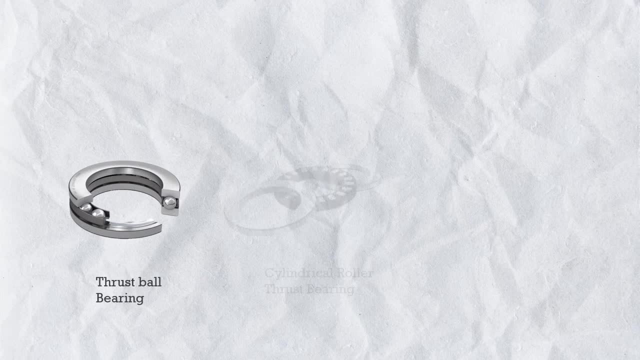 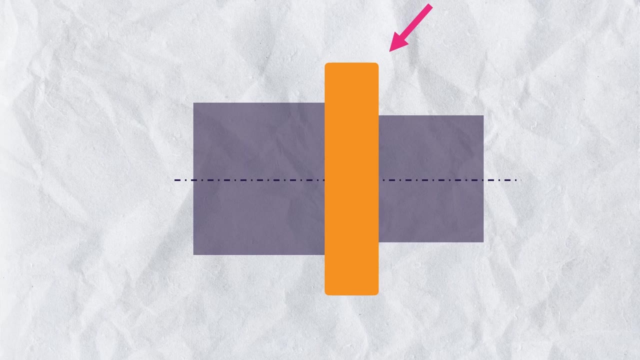 pure radial load, we used radial bearing and for the pure axial load we used thrust bearing. but as we know, in many applications load can be at some angle also or the load can be combined. load means the pure radial and pure axial but at the same time. something like this, but as per the 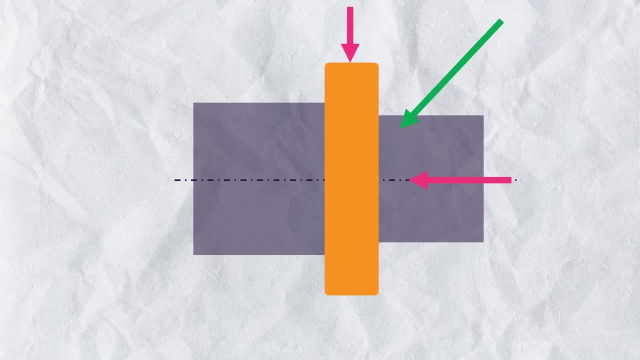 physics and vector. this is the same thing because the result can be different depending on the weight of the bearing. so, for example, if the bearing is at some angle and the load is at some angle, the rolling element of the bearing, which is ball- in this case the ball's contact line, or we can 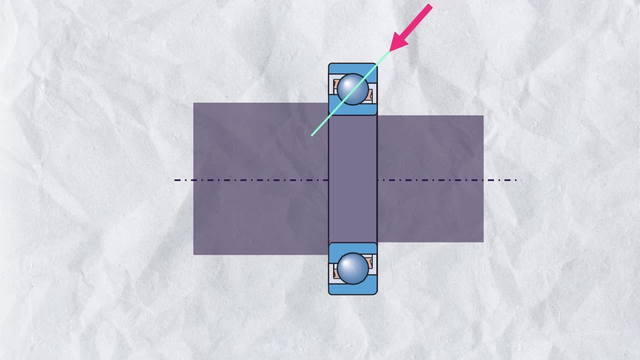 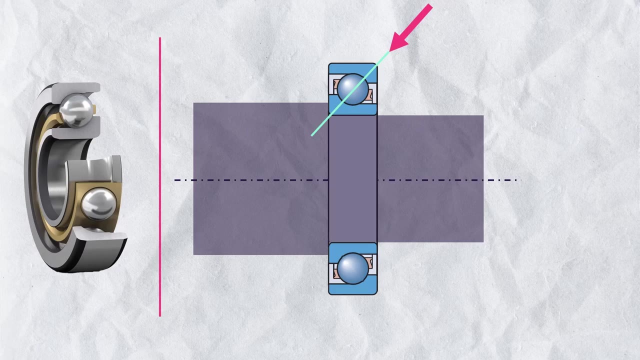 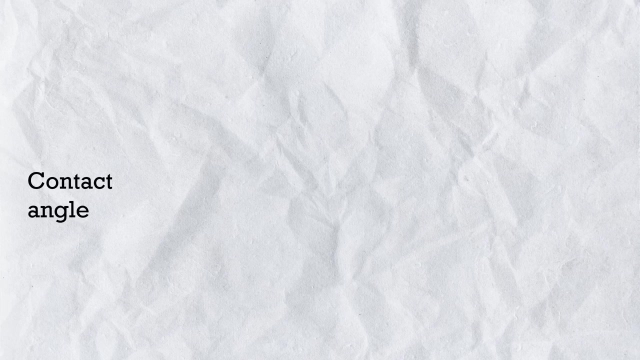 say, load line also should be at angle to support the load better, something like this, and we call this bearing angular contact, ball bearing, and this is the main feature of all types of angular contact bearings. so the first thing is the contact angle. so the standard single row angular contact bearings comes in different contact angles like 25 degree, 40 degree and in. 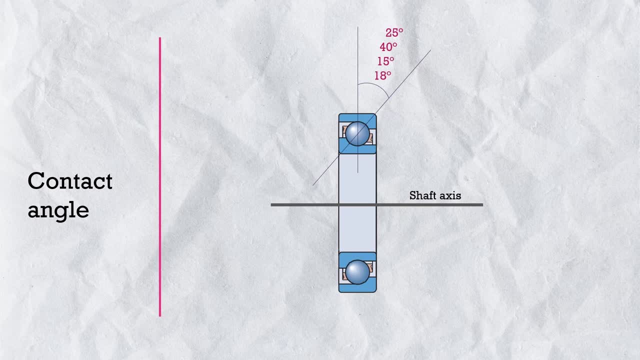 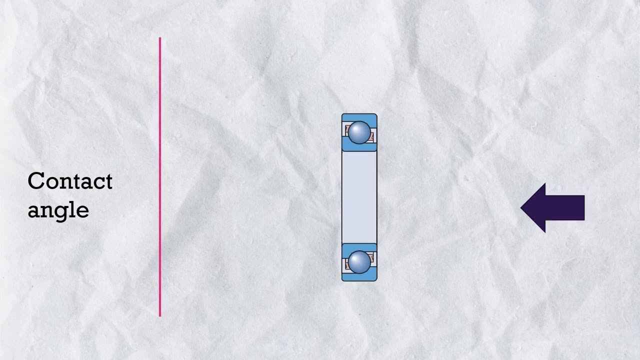 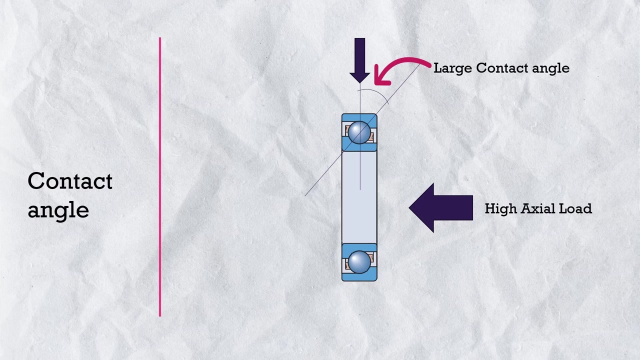 the super precision grade, there are also 15 degree and 18 degree, so which angle of angular contact bearing we should use. so it's very simple: if our application is subjected to high axial load as compared to radial load, select a large angle angular contact bearing because when contact 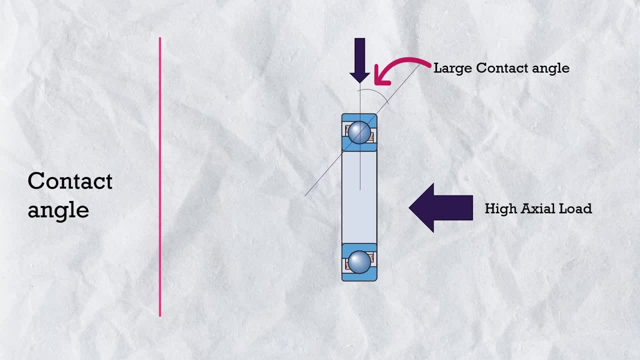 angle is large, the bearing axial loading capacity will be very high and the load capacity will be high, but radial loading capacity will be low and we also call it thrust angular contact bearing, like 40 degree angle angular contact bearing, and if our application is subjected to high radial load, 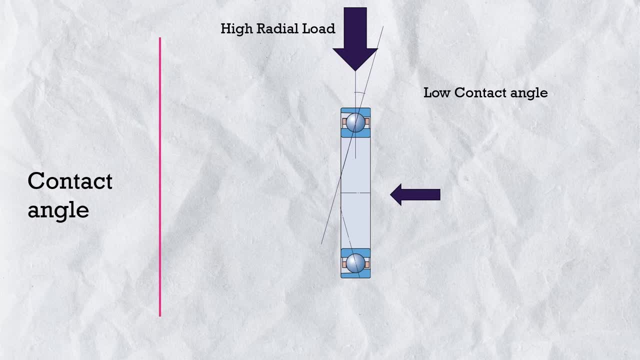 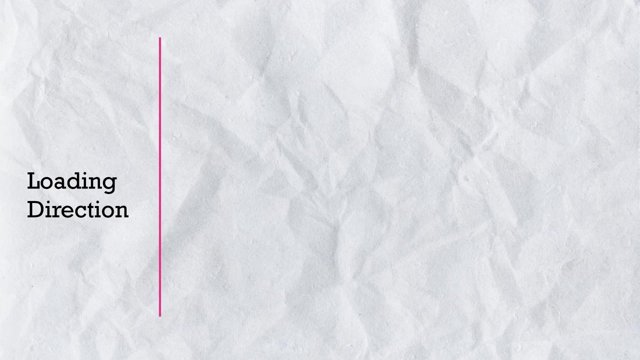 as compared to axial load. select low angle angular contact bearing because the contact angle is low, bearing radial capacity will be high, but at the same time the axial loading capacity will be low. and now the next thing is the loading diagram. so a single row angular contact bearing can take higher load in radial direction as compared to. 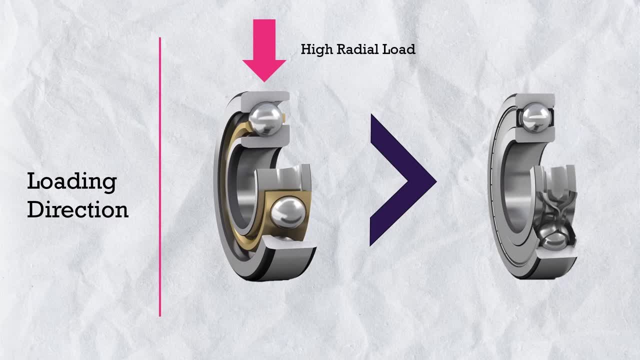 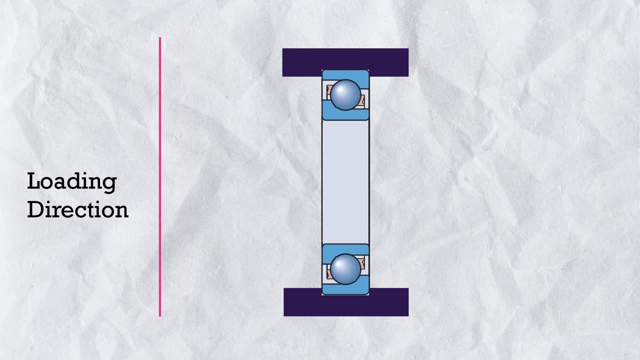 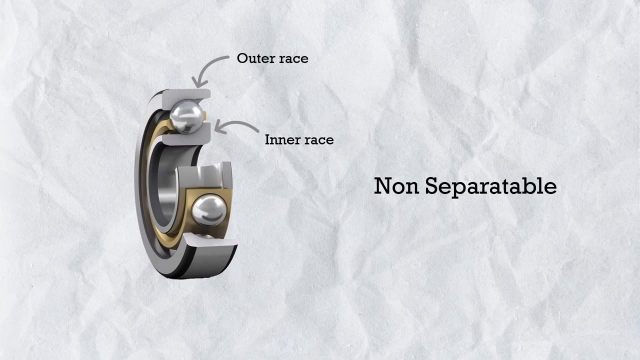 deep groove ball bearing, because this design allowed to fill more balls between the rays during the bearing assembly process. but a single row angular contact bearing can axial load only in one direction. however, angular contact bearing is a non-separatable bearing. but what if, in application, the axial load is from both side? 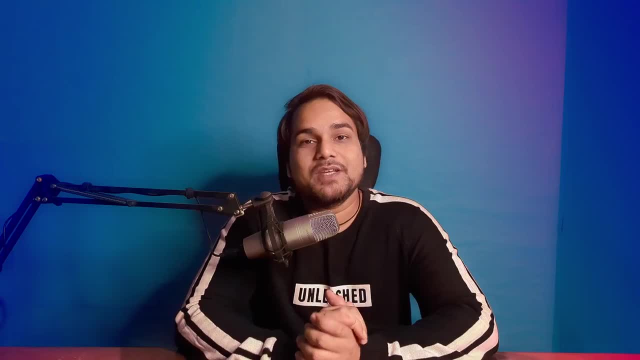 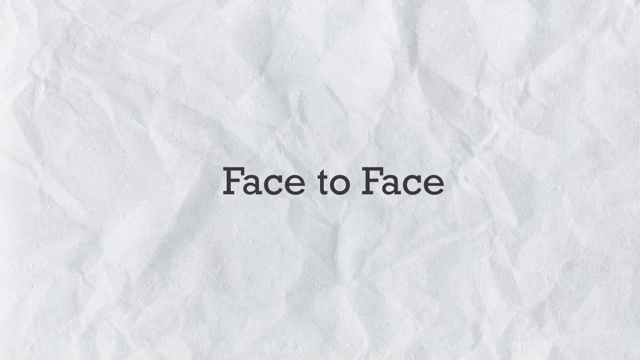 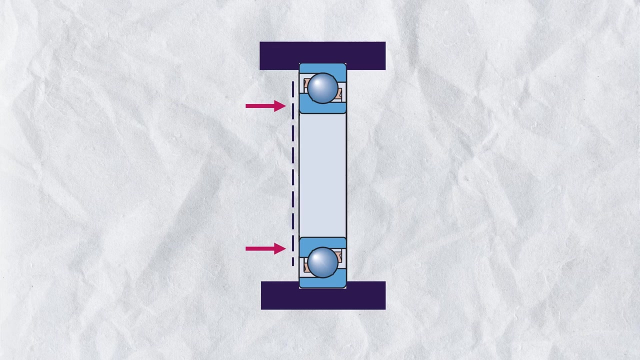 then we use pairs of angular contact bearings. and we can arrange the pairs of angular contact bearings in three possible basic orientation. the first is face to face. so which side is the bearing face? the loading side is the face of bearing. like we can apply the axial load in a shaft only in. 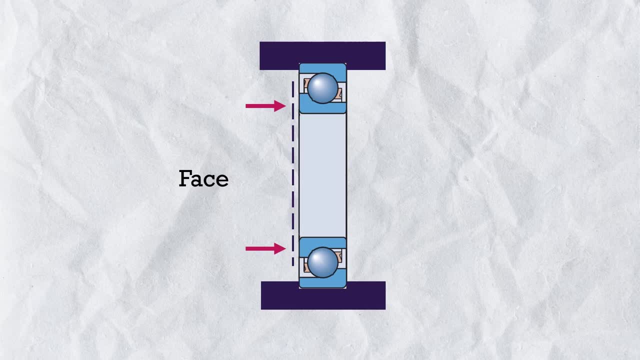 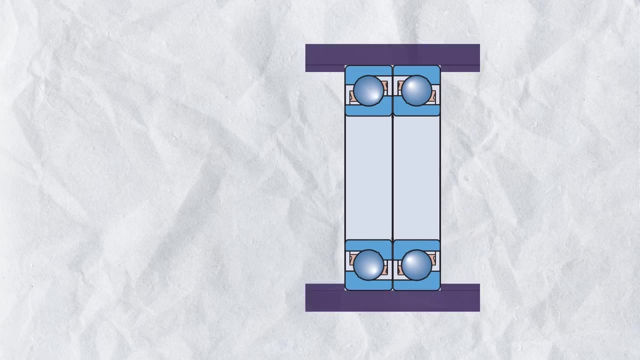 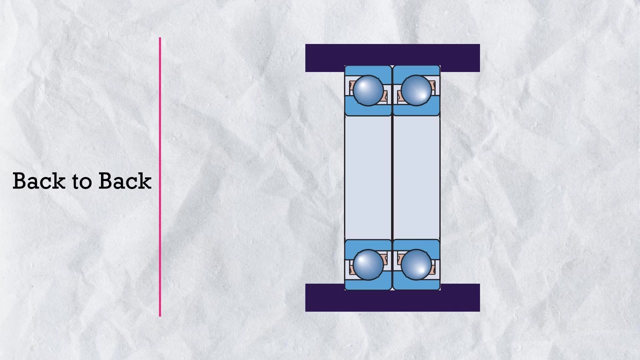 this direction. so this is the face of the bearing and opposite it's the back of the bearing. so if we put the bearing face to face, it's face to face arrangement. and if we flip, the orientation of both bearings means back to back arrangement. and if we arrange the bearing back to face, 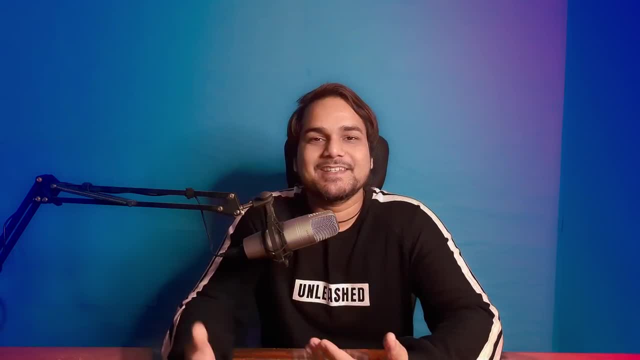 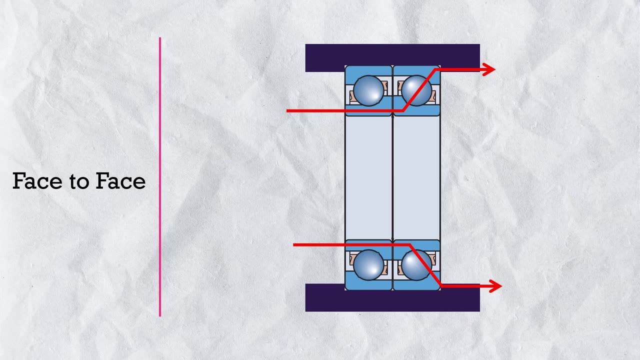 we call it tandem arrangement. and now let's understand one by one. so in face to face bearing arrangement, axial load will be transferred through only second bearing, no matter load is applied from left side or right side, something like this. so we call the second bearing active and the first. 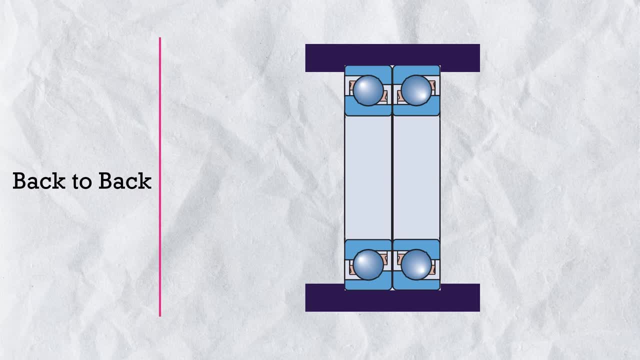 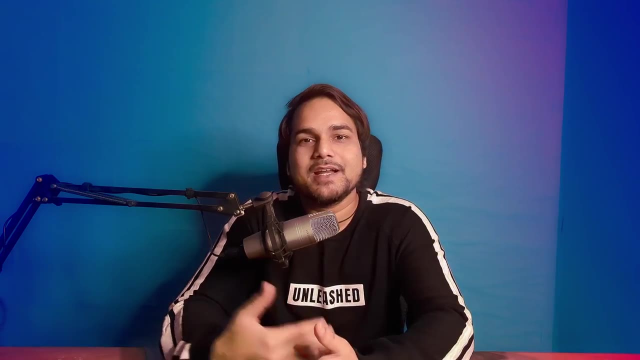 bearing is inactive and in back to back arrangement, axial load will be transferred through only first bearing, something like this: so in back to back arrangement, first bearing is active bearing and second bearing is inactive. and what about tandem arrangement? so in this arrangement, axial load will be transferred through both bearings. in this arrangement, axial load will be transferred through: 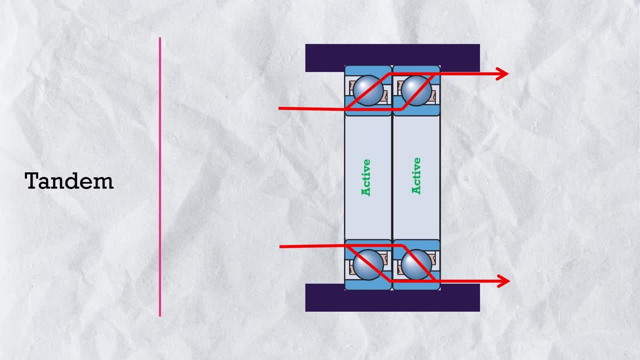 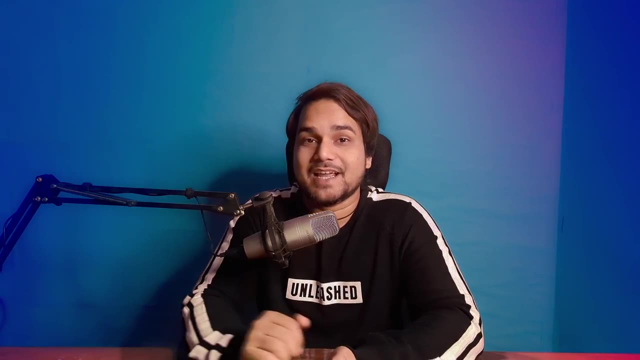 through both bearings. both bearings are active bearing, but only in one direction. in another direction bearing will not transfer the load. both are inactive. so we use the tandem bearing arrangement where load is being applied from only one direction, or we can add one more bearings with tandem arrangement in. 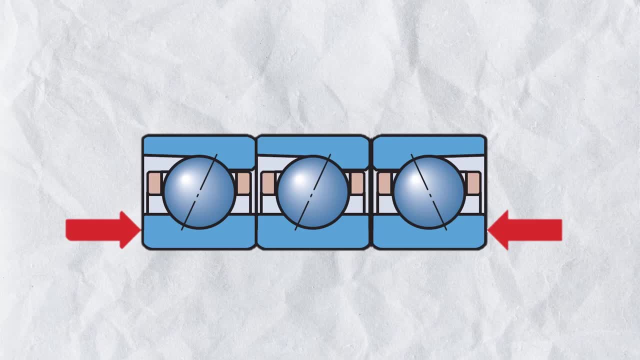 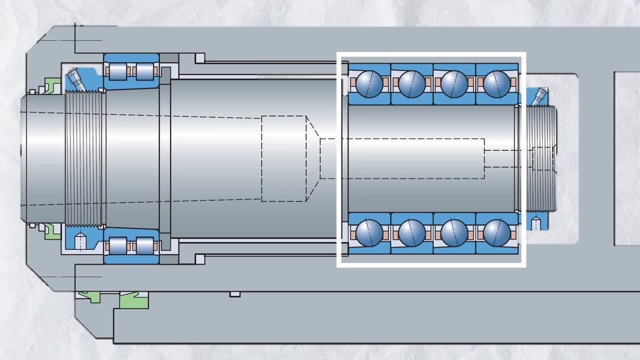 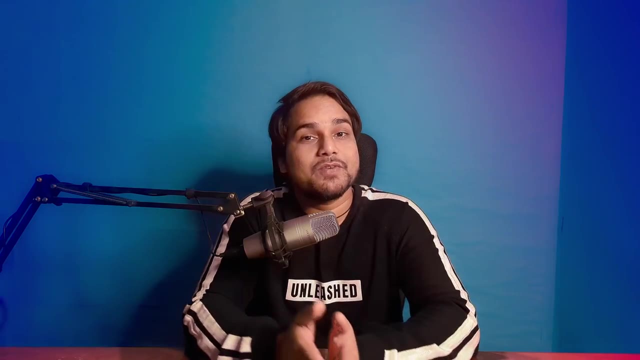 opposite orientation to support the load in another direction also. and we can use multiples bearing in one bearing block to support the heavy load and minimize the vibration, for example in ball screws support bearing unit. but you can ask as we have seen in face-to-face arrangement and back-to-back arrangement in both. 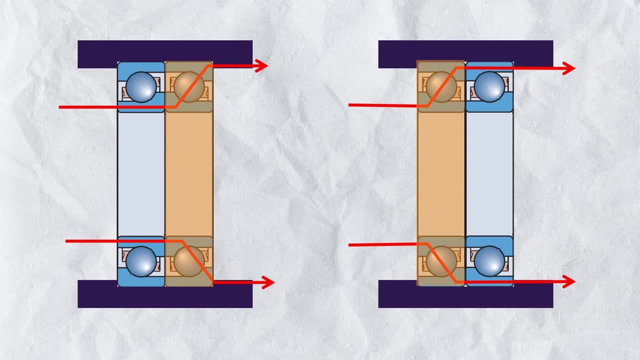 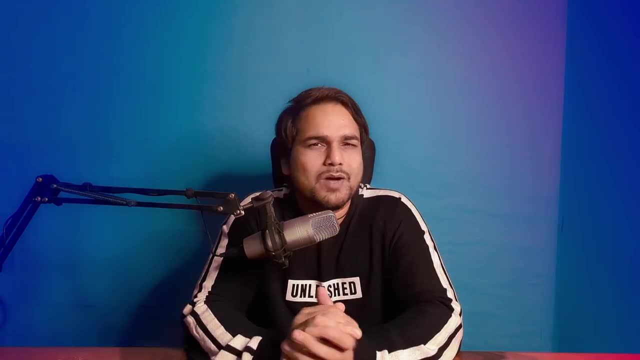 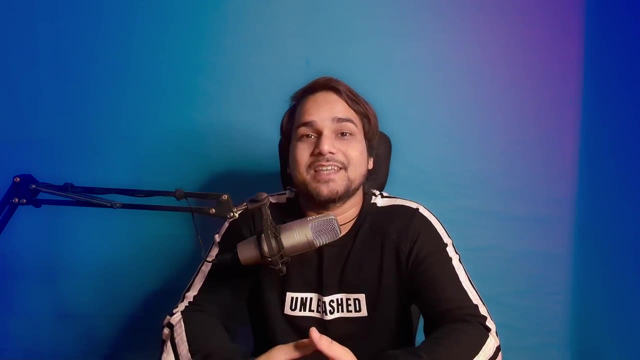 bearing arrangement. only one bearing work at the time against the axial load in a direction. so what is the difference between both bearing arrangement or why we should care about selecting right bearing arrangement, because both organism works more or less same. so the main difference is here when we extend the load line in both. 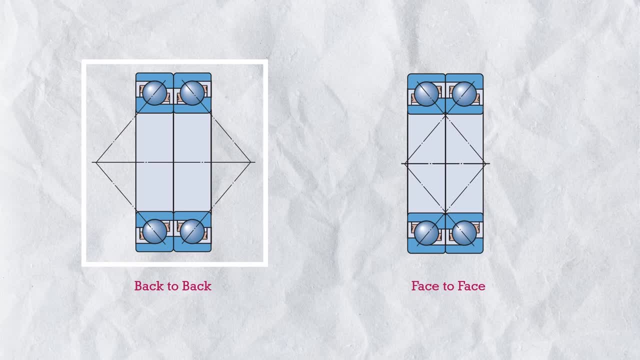 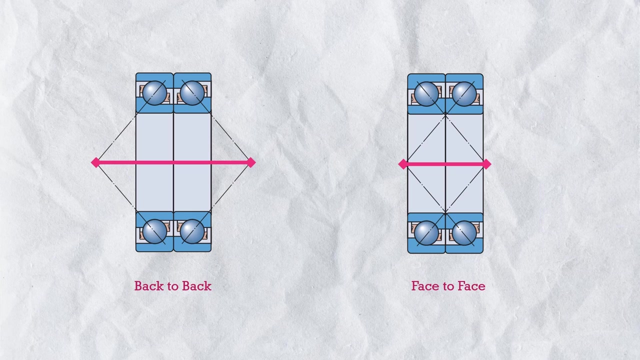 bearing arrangement. in back to back arrangement lines are diverged and intersect at a wide span as compared to face-to-face arrangement. because in face-to-face bearing arrangement load lines are converged and intersect at narrow span and this wide span between effective center mark makes back-to-back arrangement overall more rigid as compared to face-to-face bearing. 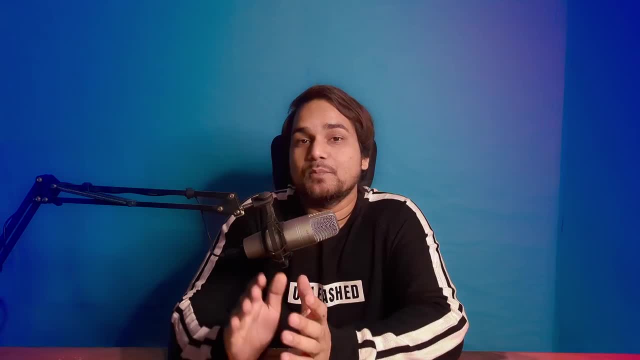 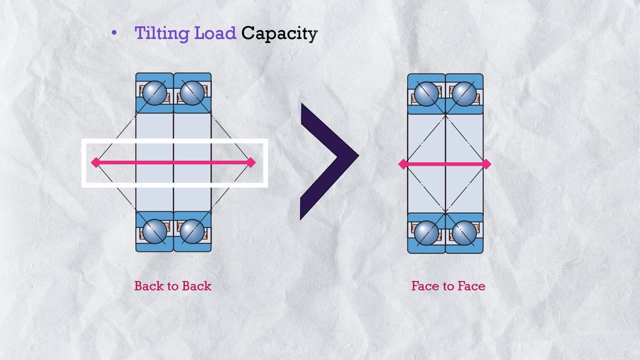 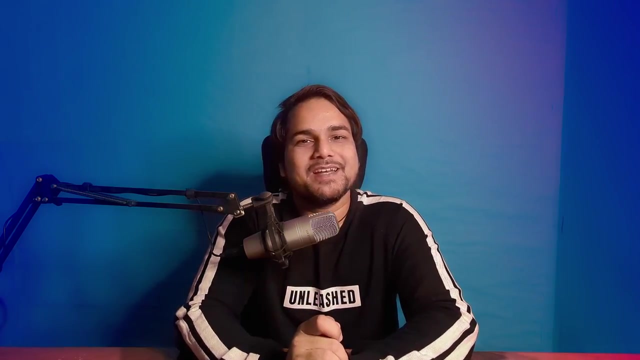 arrangement. more rigid means more stiff, and more stiff means less deflection under loading. also, wide span effective center mark makes back-to-back bearing arrangement more suitable for tilting loading. so should we always use back-to-back bearing arrangement? answer is no, because, as face-to-face arrangement are less 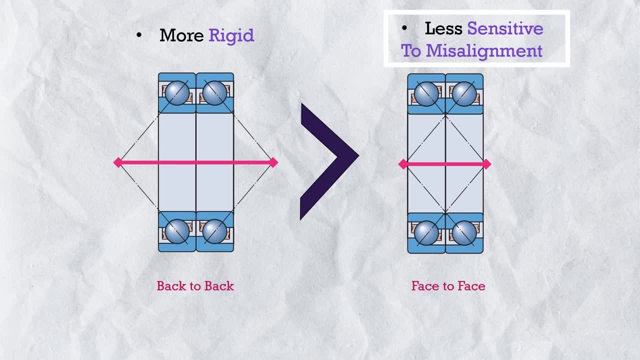 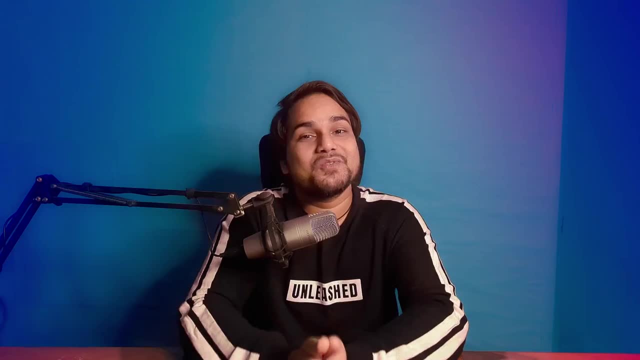 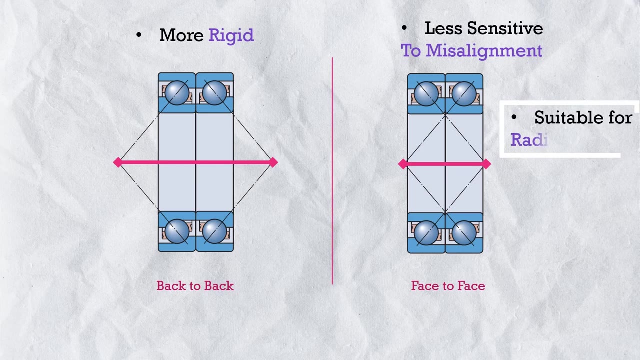 stiff and more rigid as compared to face-to-face bearing arrangement. effective arrangement: it means face-to-face bearing arrangement are less sensitive to the misalignments. it means face-to-face arrangement can give more service life in misalignment condition as compared to back-to-back arrangement. second, face-to-face arrangement is more suitable for. 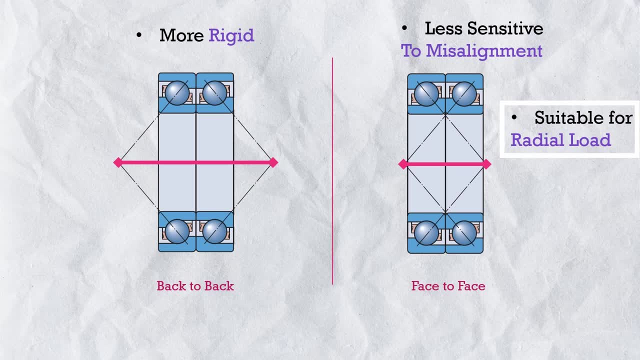 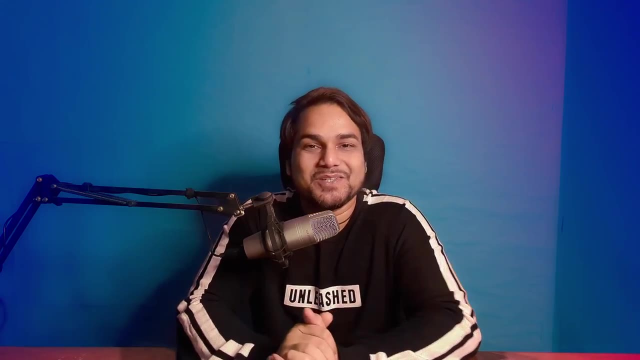 radial loading condition as compared to back-to-back arrangement, and back-to-back arrangement is more suitable for axial loading, but face-to-face arrangement is more suitable for managing bending movement as compared to back-to-back arrangement. So much confusion, so let's summarize it for the selection purpose, for the easy selection. 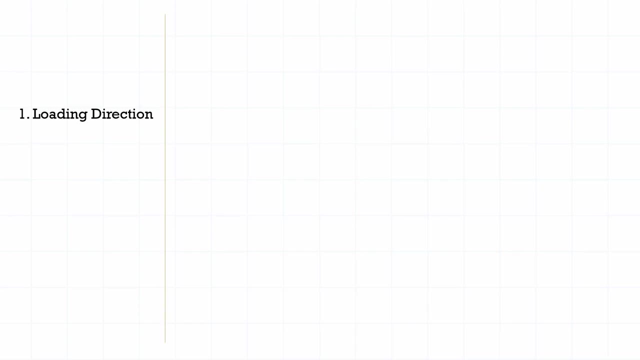 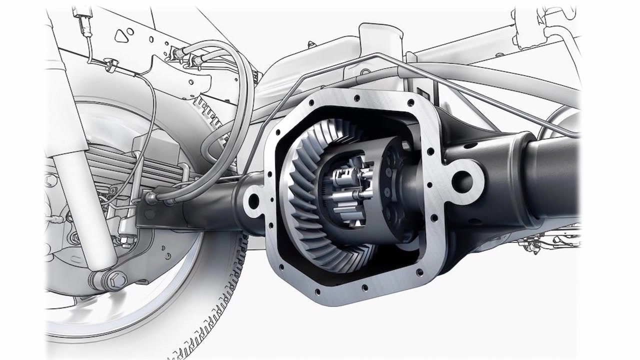 purpose: 1. The loading direction In application where axial load, or we can say thrust load, is primary, or maybe we need precise control over positioning in axial direction. go with the back-to-back arrangement, For example car differential or milling machine where we apply high thrust load during material. 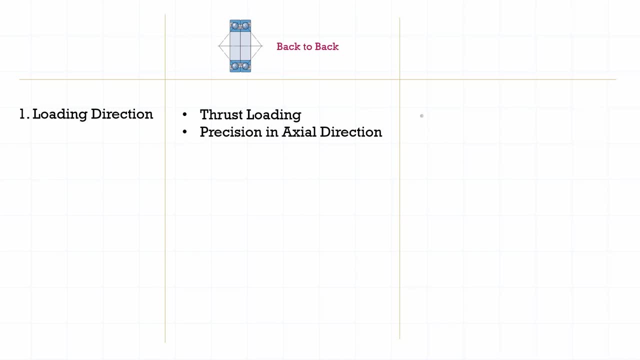 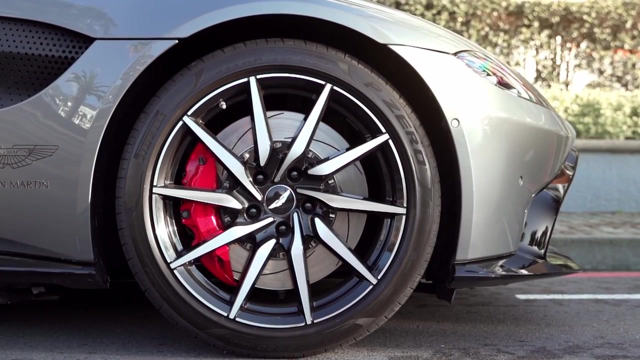 cutting, material drilling and the application where radial load is primary or maybe you need precision control over positioning in radial direction. go with face-to-face arrangement like electric motor car wheels bearing hub. the radial load is dominating because of weight of the car.